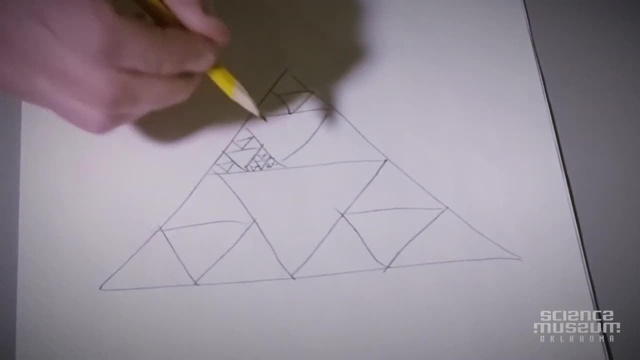 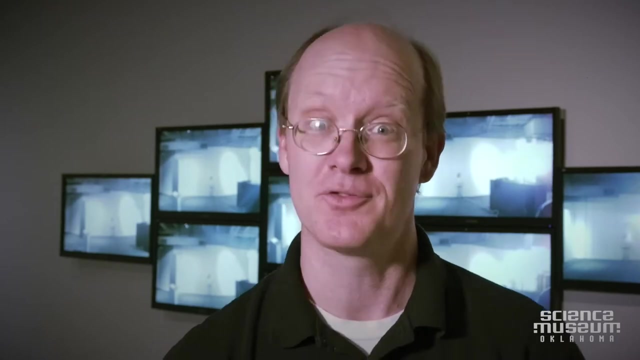 get your magnifying glass and a really sharp pencil. you can keep going and keep going, and keep going until your pencil isn't sharp enough to go anymore. That is a fractal Science Museum. Oklahoma, with the support of the Oklahoma Arts Council, is bringing you an exhibit right. 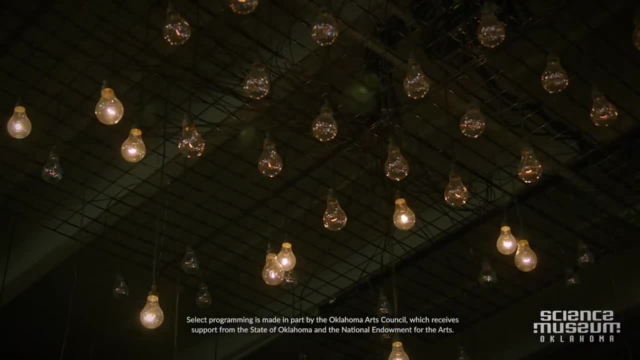 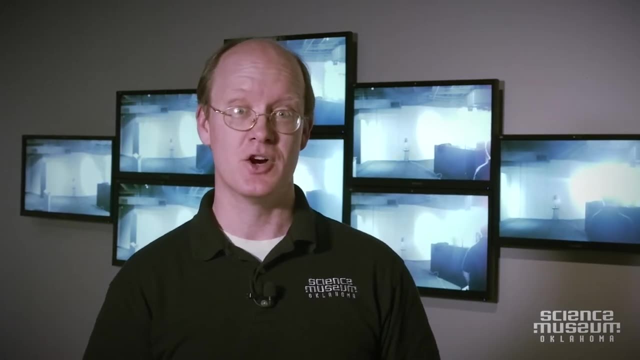 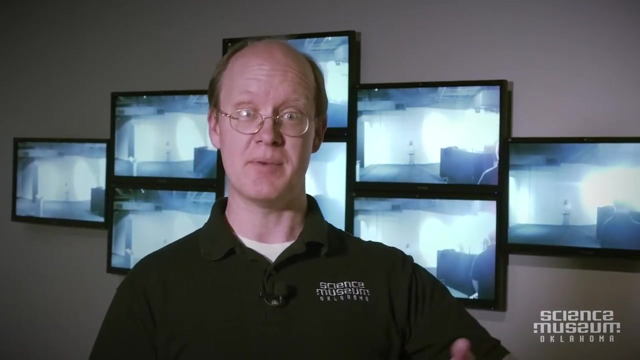 now called Screens by Jeffrey Hicks. It uses a lot of screens and other technology, like cell phones, that I'm going to show you today, to create some beautiful art. So the art that we have with fractals uses art and mathematics. It was actually created by a guy named Mandelbrot, a mathematician, And 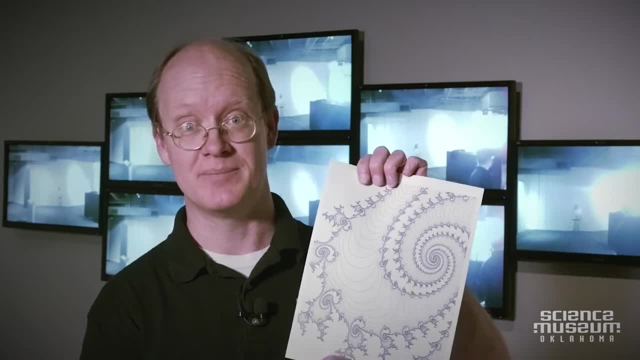 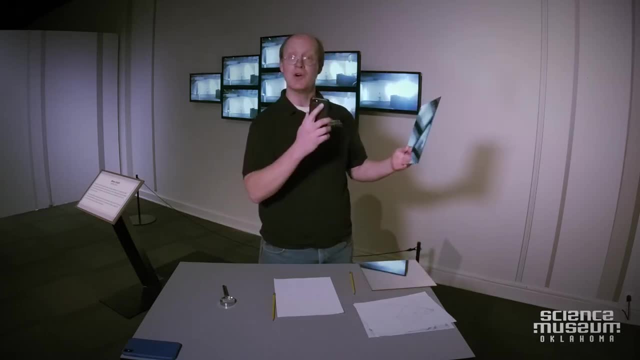 some of these pictures are beautiful, like this one. Well, here's one more. you can try: If you've got your cell phone and you've got a mirror, you can point your cell phone, set it on cell phone and you can use it as a mirror. You can point your cell phone, set it on cell. 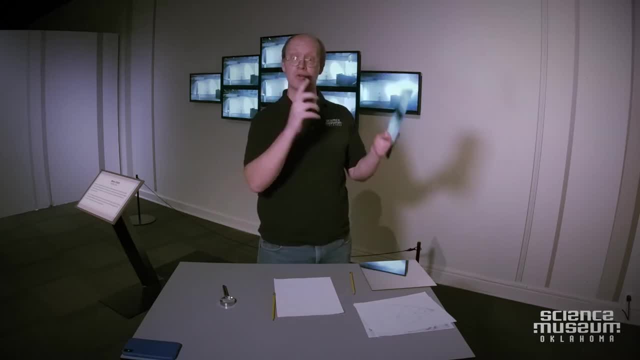 phone, set it on selfie mode, point it at the mirror and you see the image of the cell phone in the mirror. Or if you get two cell phones, it's really cool. So you point one cell phone at the other cell phone, put them both on selfie mode and this cell phone shows. 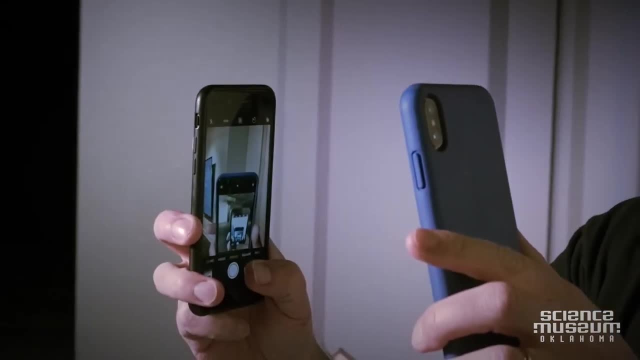 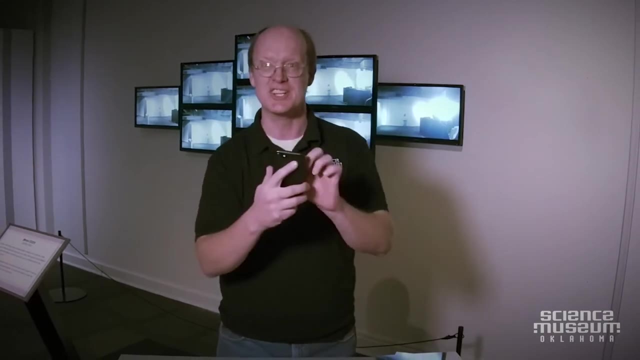 you a picture of this cell phone. This cell phone's image has this cell phone in it, which then has this cell phone's image and this cell phone's image, going on and on and on. Snap a picture and then start to zoom in and you see, the cell phones continue well, until. 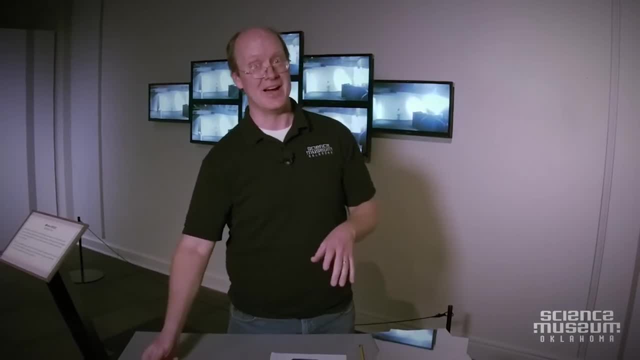 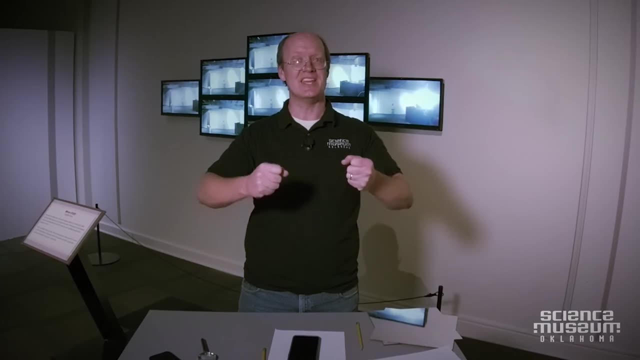 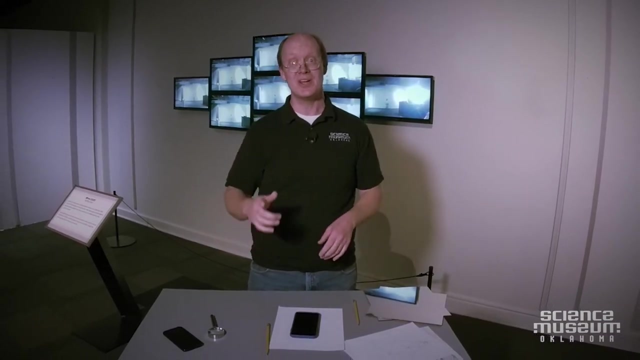 the pixels are too small to see another one. It's kind of cool. Now, the beautiful thing about mathematics and art is mathematics allows us to explore the infinitely small or the infinitely large things that we can't see in our normal experience. And so try one of these fractal art things, explore some of them, look at them with magnifying. 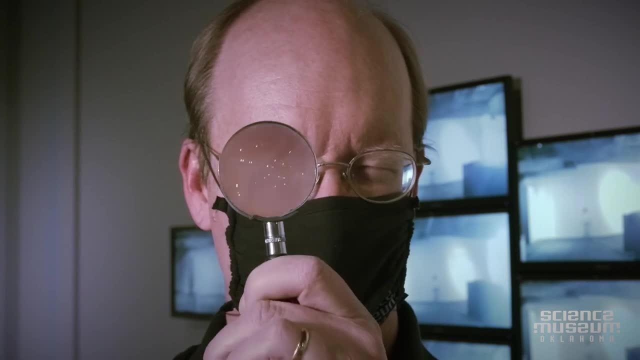 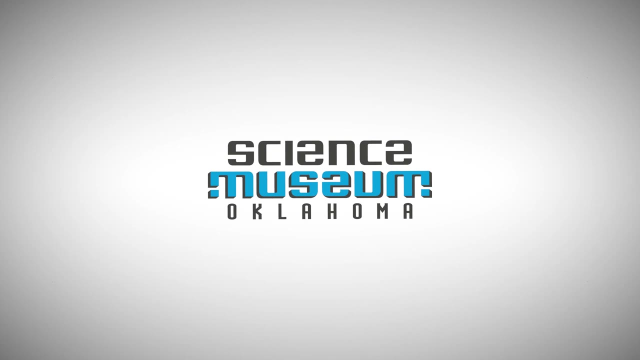 glasses, and let your imagination soar all the way to infinity Captions by GetTranscribedcom.